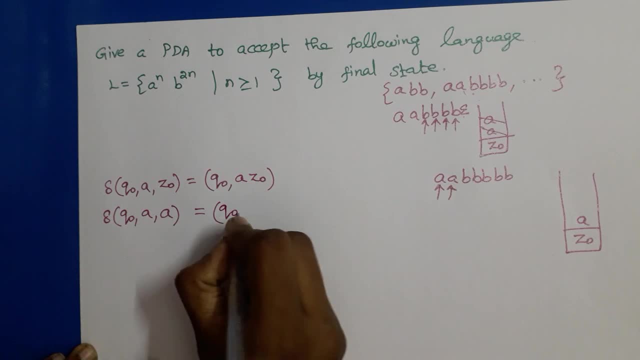 So We should remain in the same state. q naught And we have to push another a also onto the stack. so one a should replace a on top of the stack, another a must be pushed onto the stack. so this can be represented in a diagram. 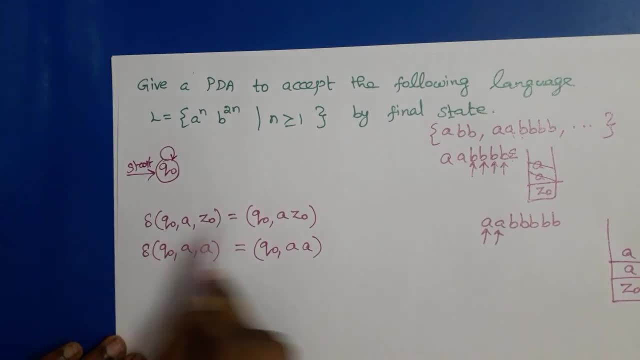 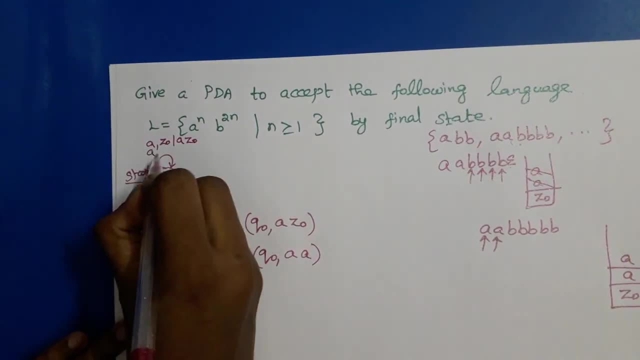 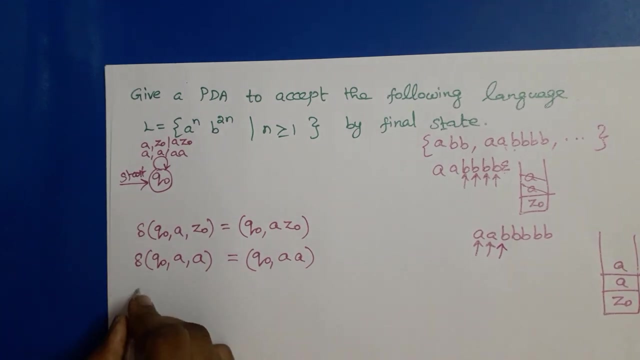 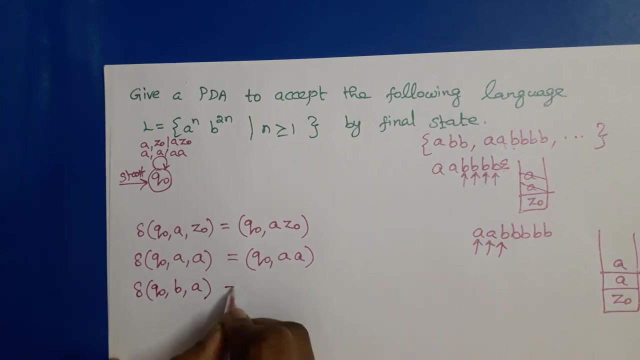 So start From q naught to q naught: a is a input, z naught is a top of the stack. a, z naught, then a comma: a, a, a. Next input is b and we are in state q naught. so delta q naught, comma, input symbol b and the top of the stack is a. so now 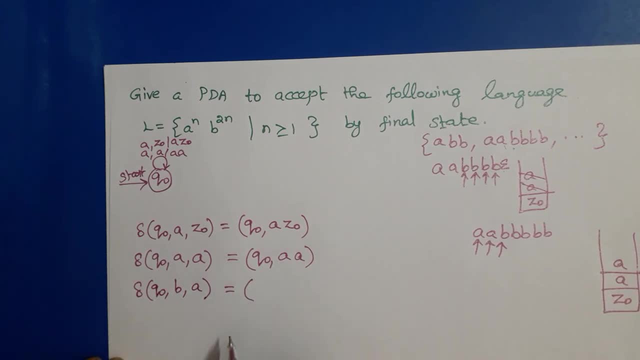 As i already told, we should not do any operation on the stack, but we have to move to the next state, q1. so state should be changed to q1. and no operation on the stack means we need to write the same symbol here, so a should be written here. 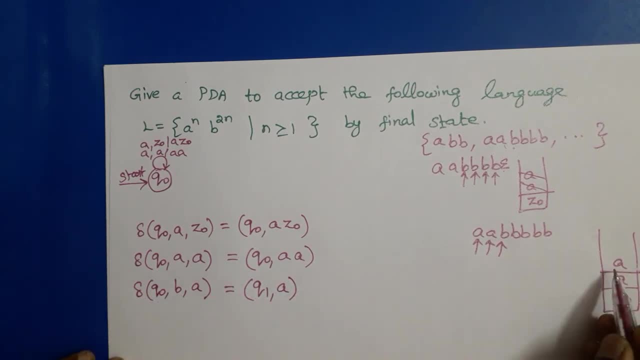 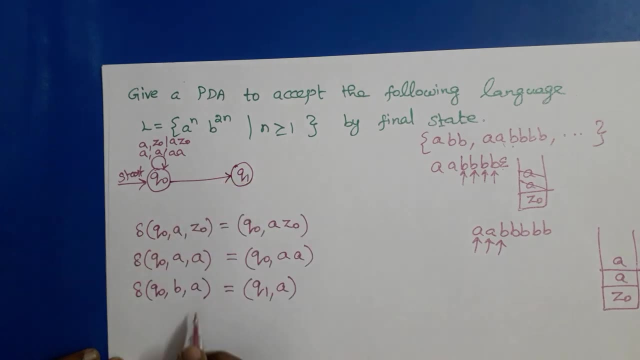 So state change to q1, no change in b, no change in a. okay, so here q naught to q1, from q naught to q1, and the h must be labeled by b, comma a, slash a. then q1 is a current state and the next input is a, and here i have written 5 b's, sorry, only 4 b's. 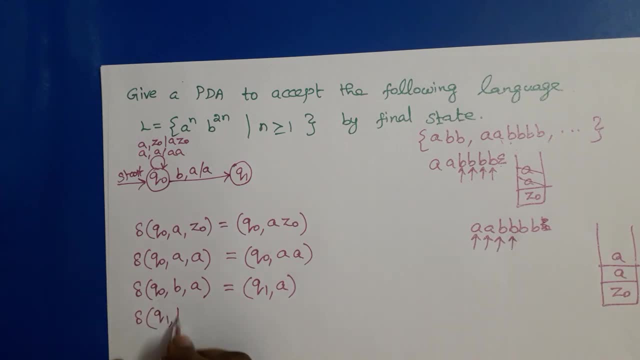 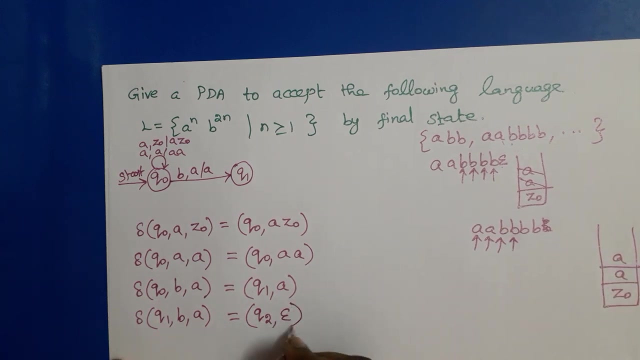 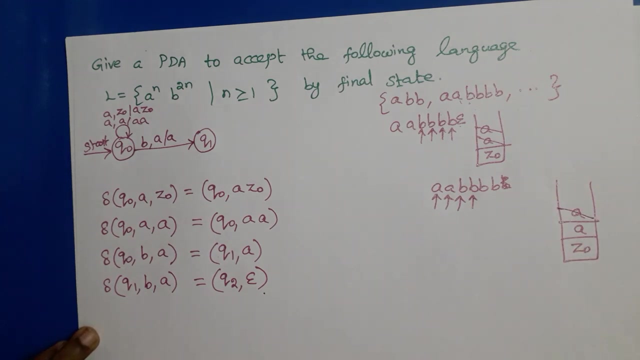 So The next input is b and the top of the stack is a. so now we need to change our state to q2.. And one a. the pop operation must be performed right, so that should be written like epsilon. the meaning is: epsilon replaces a on top of the stack. so pop, pop, the stack is performed. so q1 to q2.. 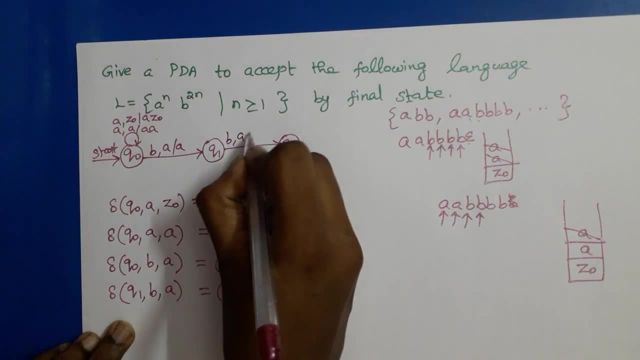 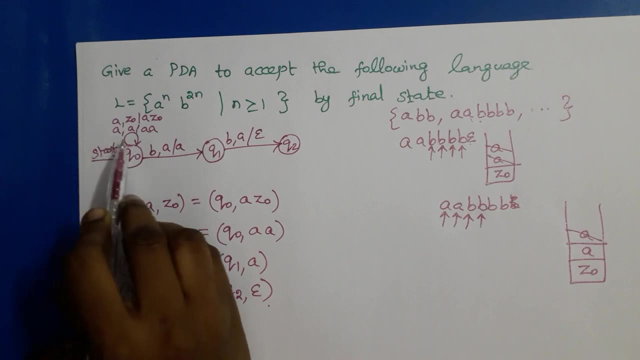 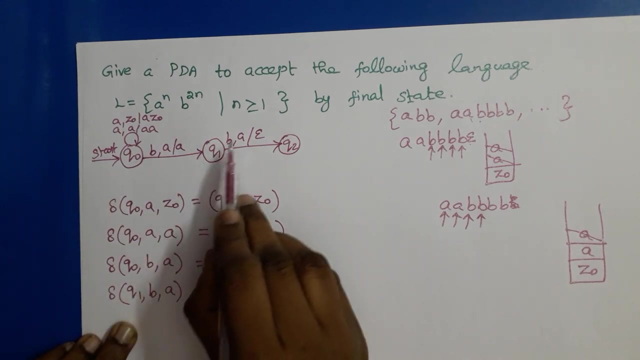 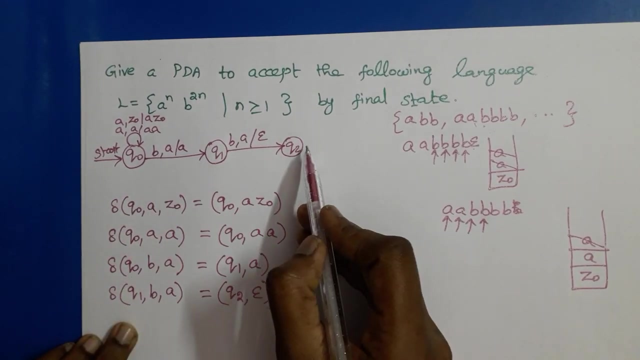 So B, comma a, slash epsilon. okay, so for the first b, For all yes, for all yes. in the input we should remain in the same state and all yes are pushed on to the stack. for the first be, no change in stack is performed and we go. we go to the state q1. for the second be, we go to the state q2. right for the third b. that is again odd number of b. for the third b. 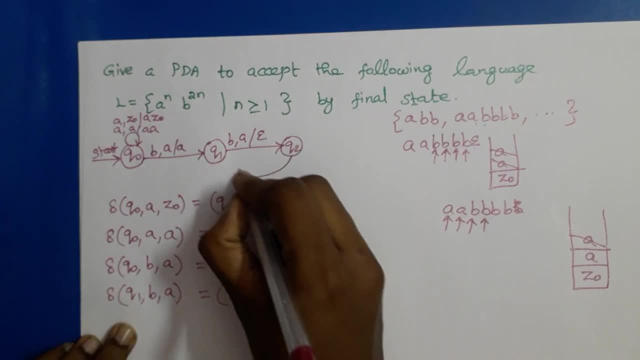 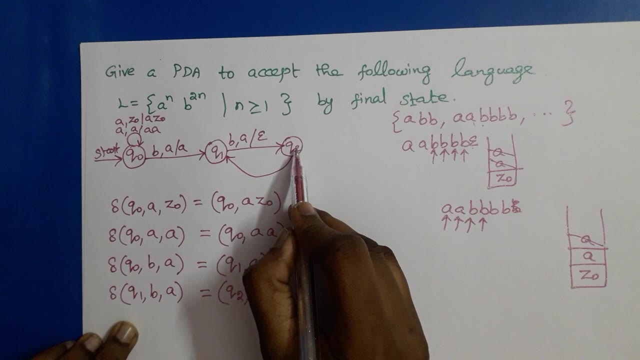 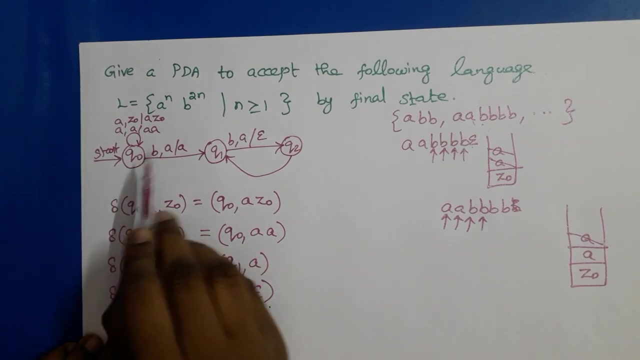 So We should go to q1, state q1 right. then only again for the second, for the fourth b, for the even number of b, we can go to the state q2.. So For odd number of b's we should be in the state q1 and for even number of b's we should be in the same in the state q2 right. so from q naught, if we see first b we have to change our state to q1. and for the second b, that is even number of b, pop operation is performed. 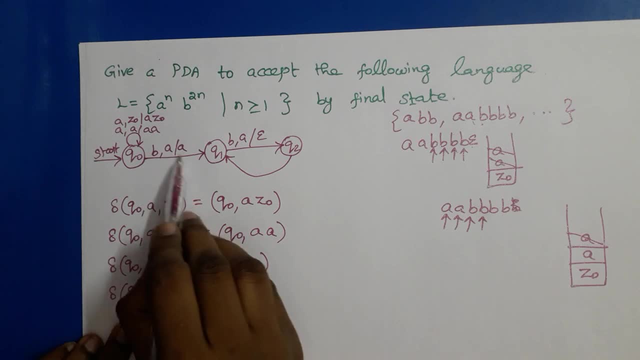 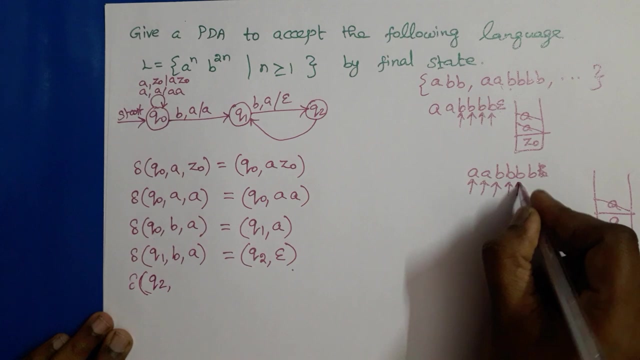 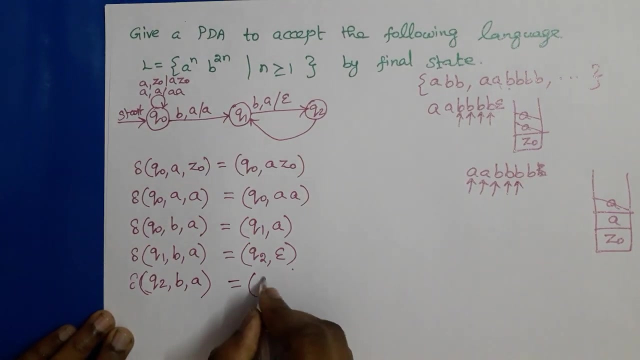 Here for odd number of b, no change operation is performed. but for the even b we have to pop 1 a from the stack. so we should change our state from q1 to q2. now we are in state q2 and the next input is b. okay, top of the stack is a means we have to go to the previous state. 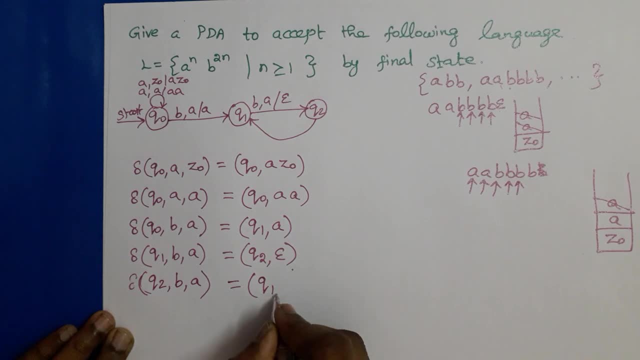 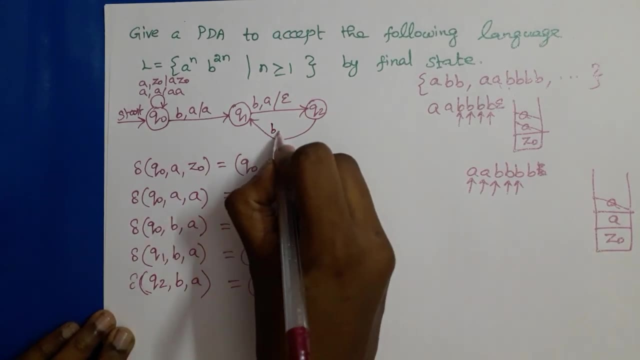 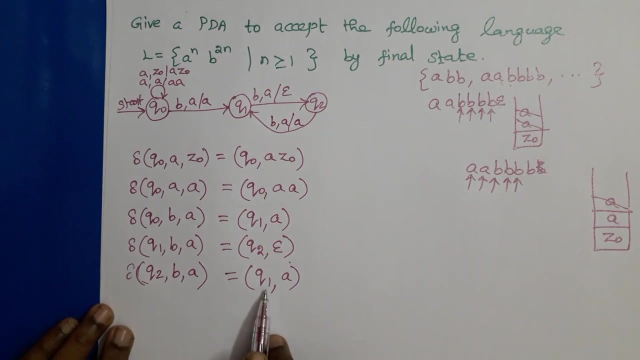 because it is repeatedly performed. so q1 comma, no change, operation. no change means we have to write a here. so q2 to q1: the edge is labeled by b comma. a slash a. okay, so now what is current state? q1? q1 is a current state and b is the next input, right? so q1 is a current state, b is the next input. 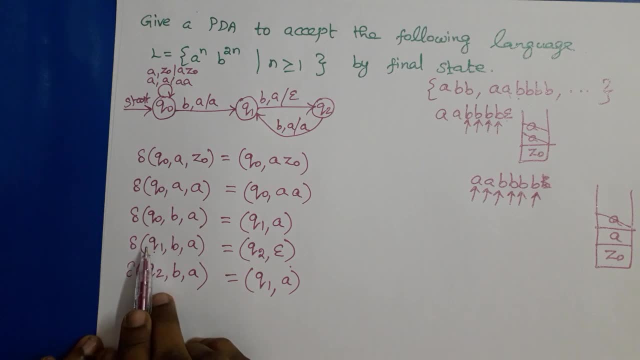 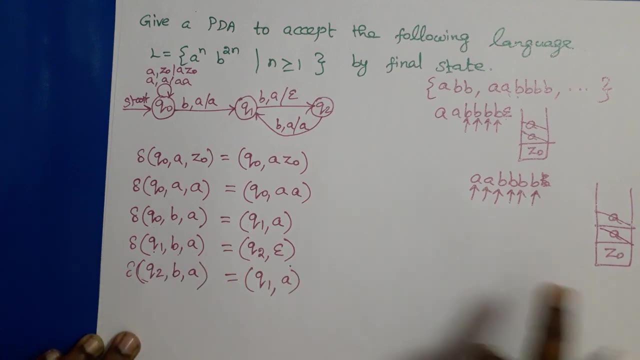 top of the stack is a. top of the stack is a means b is the next input, right, so q1 is the current state. b is the next input. top of the stack is a. we should go to state q2, and a is popped. so this is performed, okay. so now we are reading.